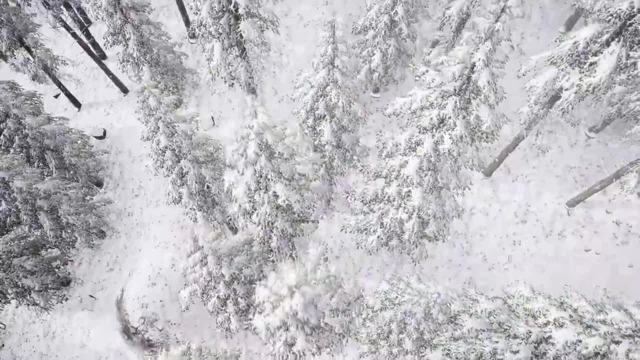 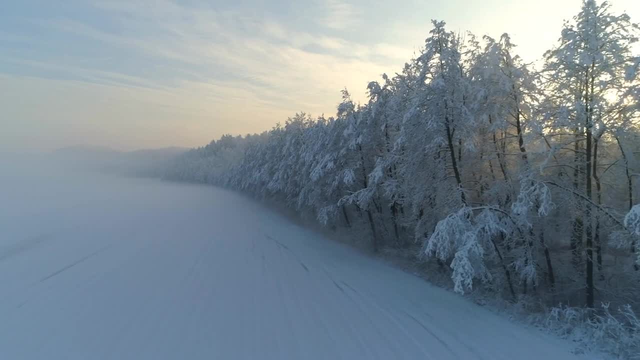 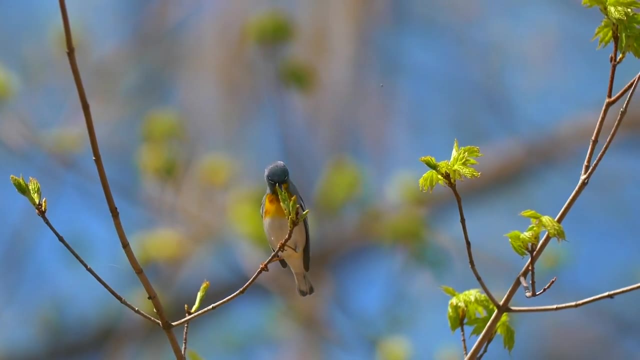 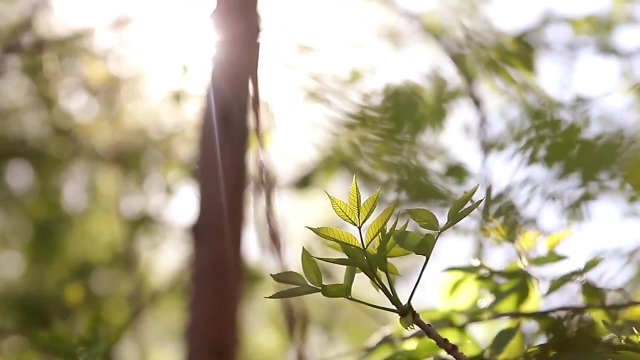 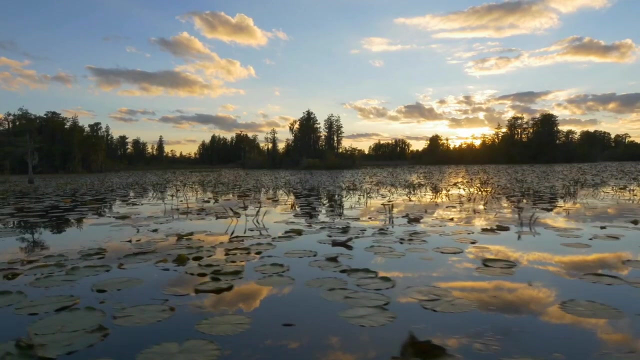 Winter is the coldest season with the fewest hours of daylight. In spring, the weather starts to warm up and the number of daylight hours increases. Each season lasts for about three months and occurs once over a period of one year. Let's take a look at the Earth and its movement around the Sun. 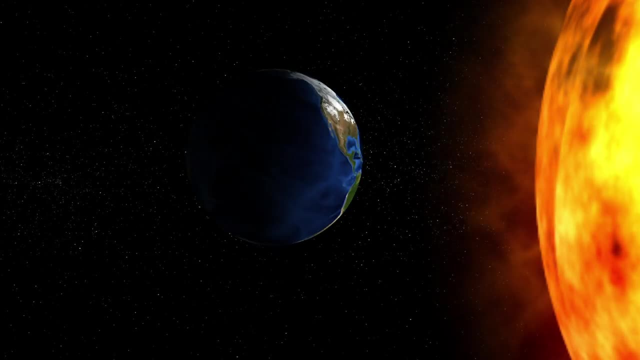 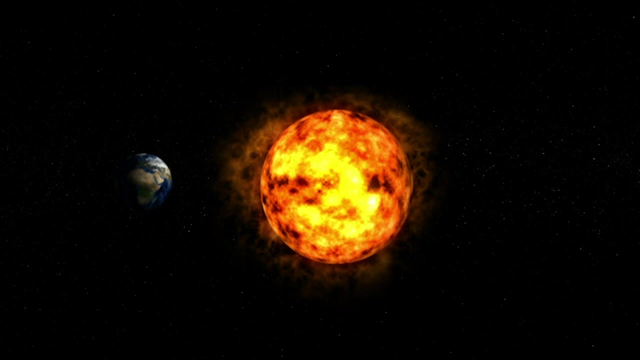 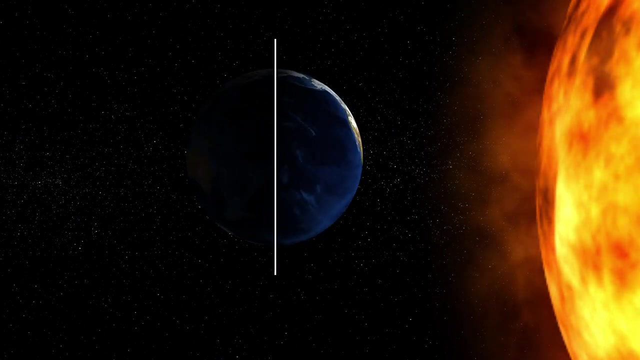 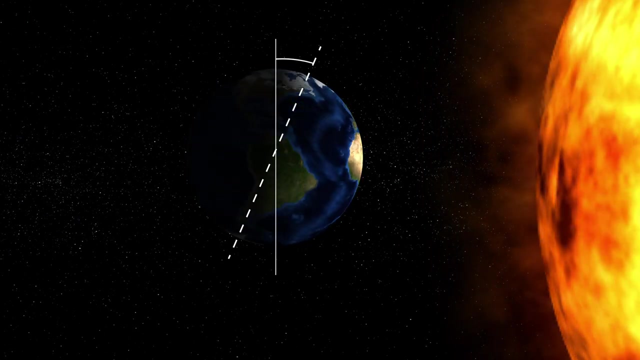 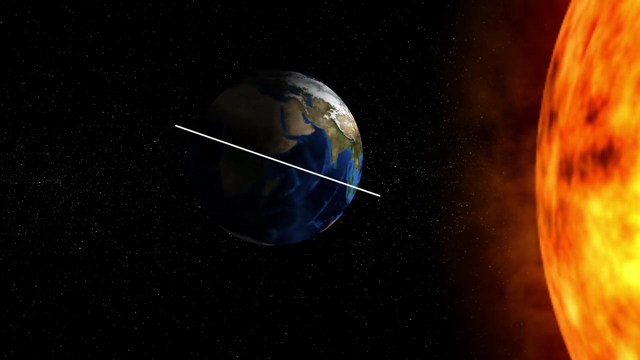 You probably already know that the Earth rotates about an axis. It also revolves around the Sun. The Earth does not rotate straight up and down. It's tilted at an angle. It's this tilted rotation that causes seasons. The Earth can be divided into two parts, called hemispheres. 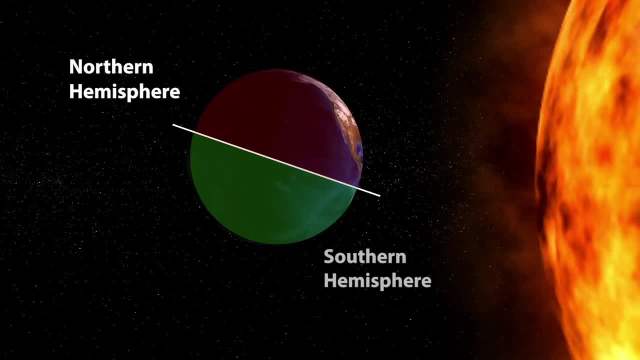 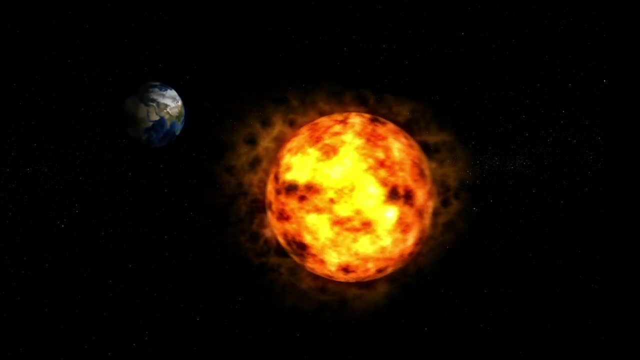 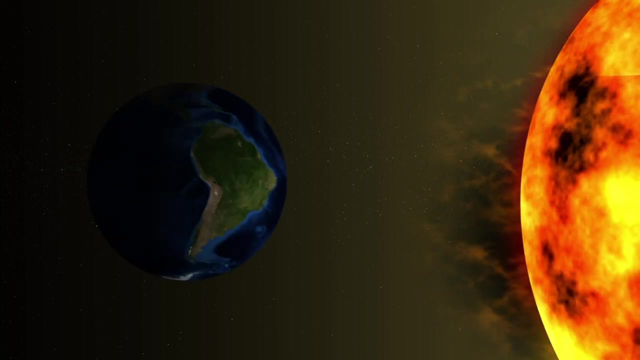 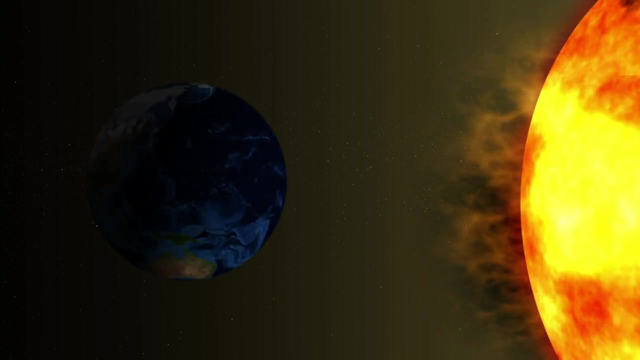 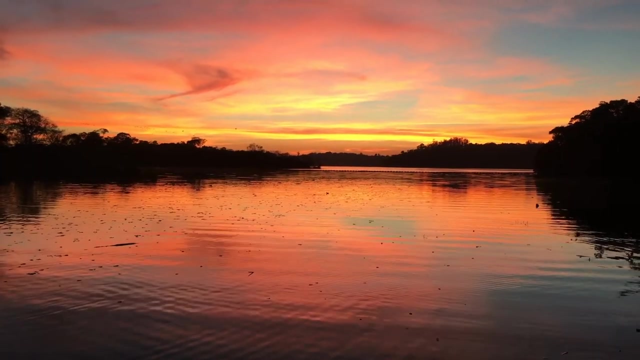 There's the Northern Hemisphere and the Southern Hemisphere. When the Earth is positioned here, the Northern Hemisphere is tilted towards the Sun. It receives more direct sunlight than the Southern Hemisphere. This results in warmer weather and more hours of daylight- It's summer. 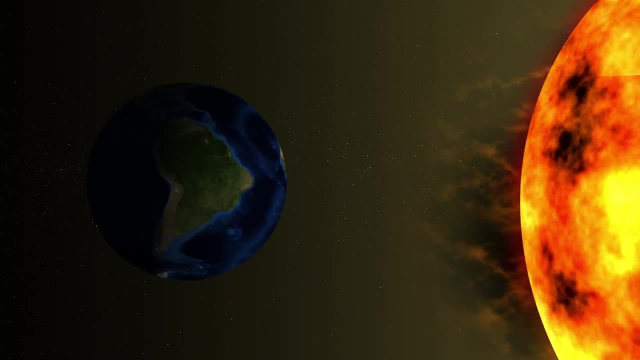 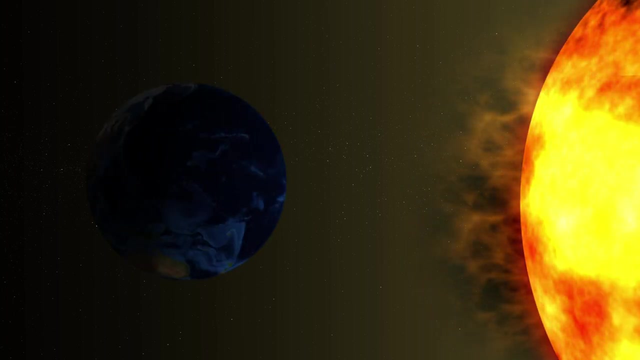 At the same time, the Southern Hemisphere is tilted away from the Sun. It rotates around the Sun. At the same time, the Southern Hemisphere is tilted away from the Sun, It receives less direct sunlight, The weather is colder and the days are shorter. 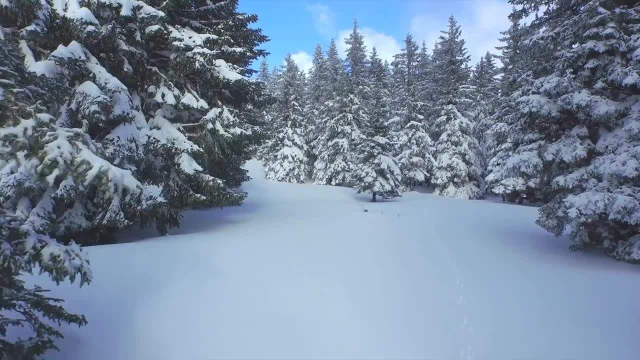 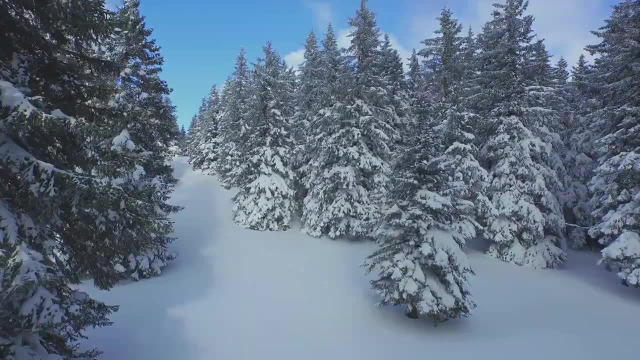 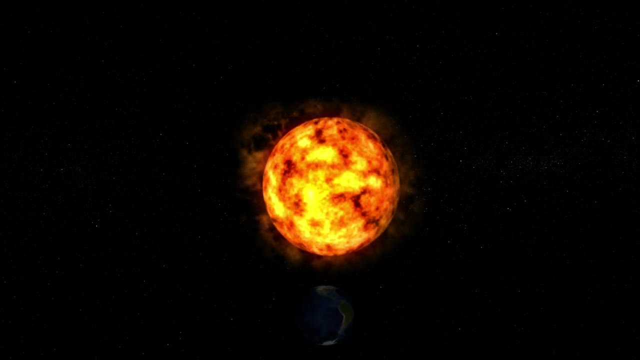